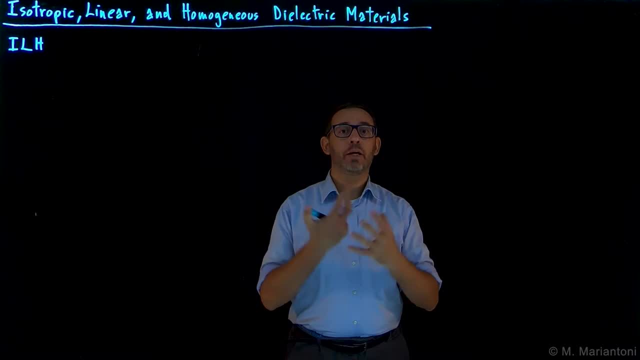 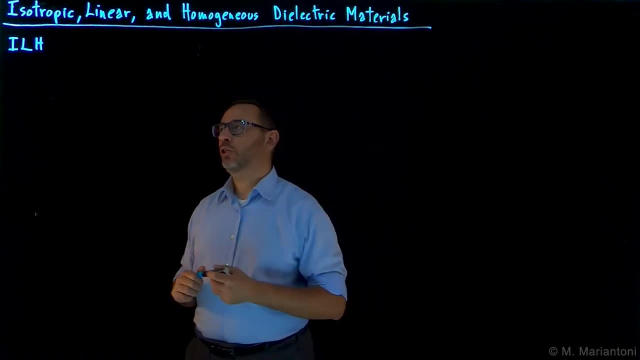 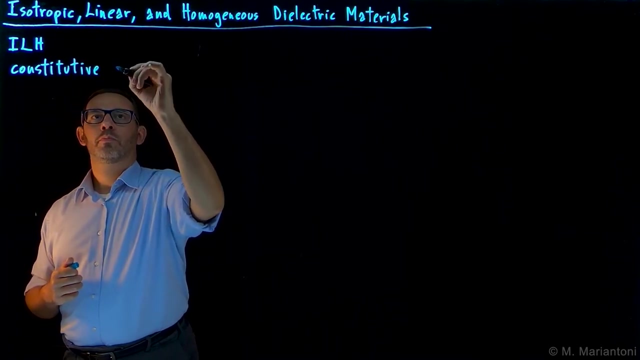 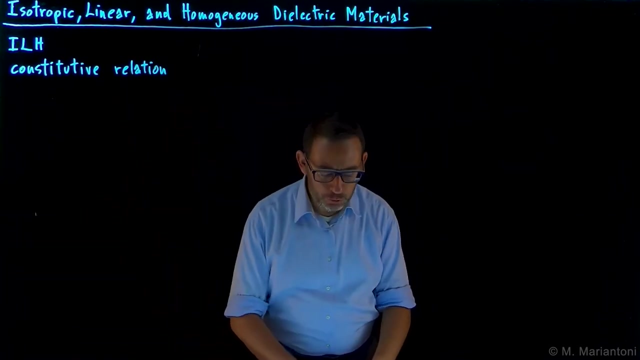 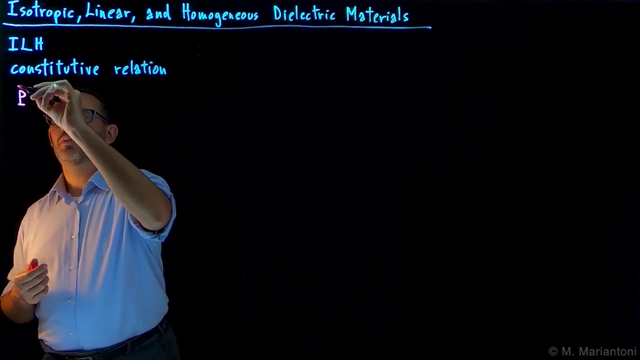 However, we need to connect these two entities, these two fields, in order to grasp more knowledge about dielectric materials. The connection between them is called constitutive relation. So what is the most general constitutive relation between four dielectric materials? Well, it's a generic function which relates the vector capital P, the polarization vector. 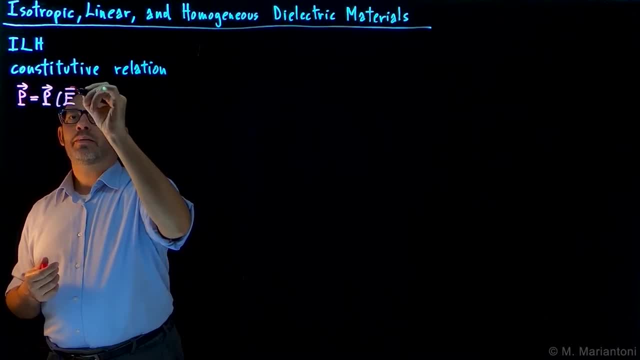 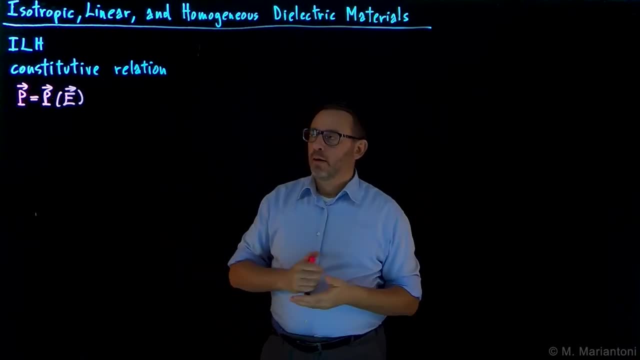 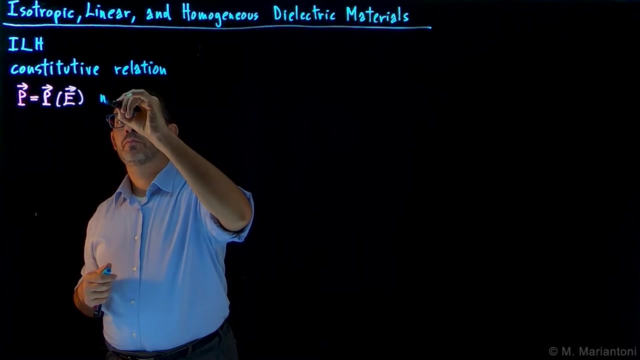 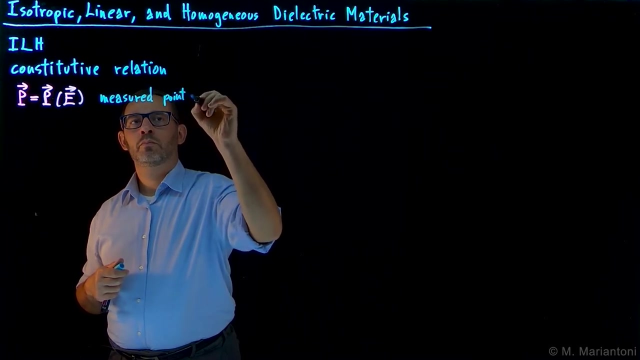 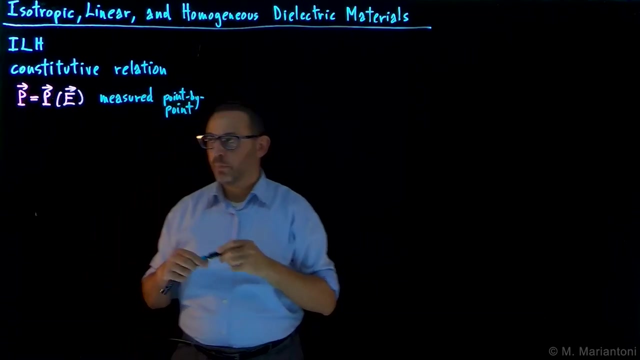 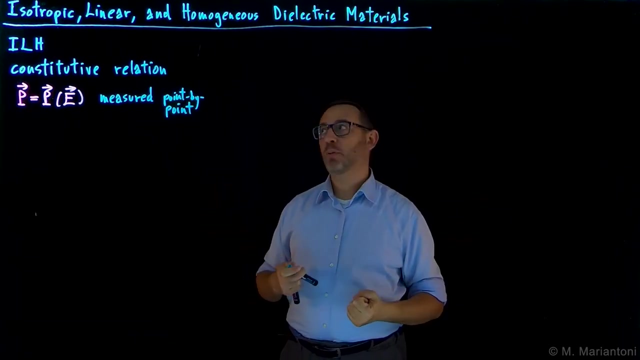 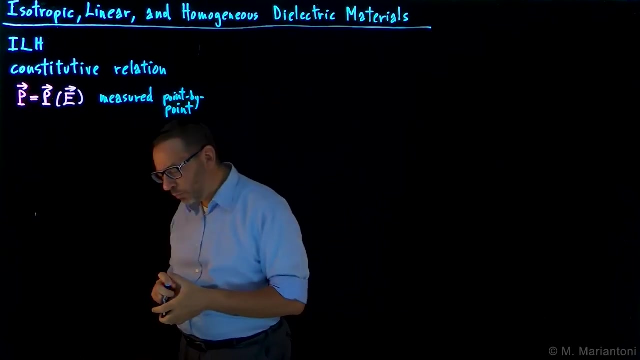 to the electric field E. So this capital P vector, function of E just means that P is function of E And these constitutive relations typically must be measured point by point Inside the dielectric material. This is a very generic function, So we want to specify a little bit more. what is the mathematical expression for this function? under certain conditions. 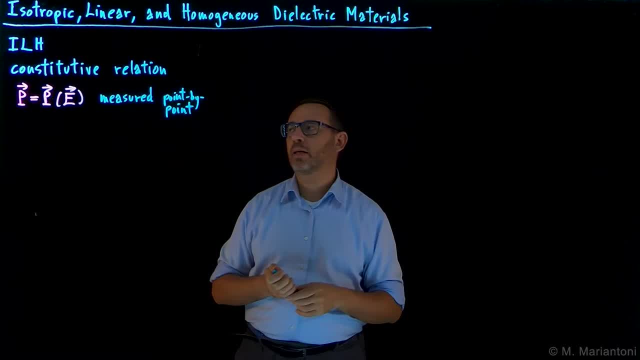 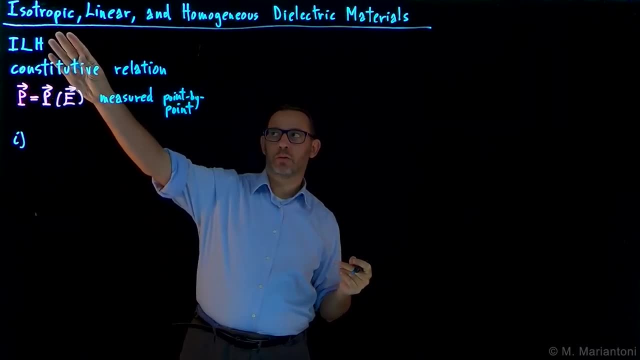 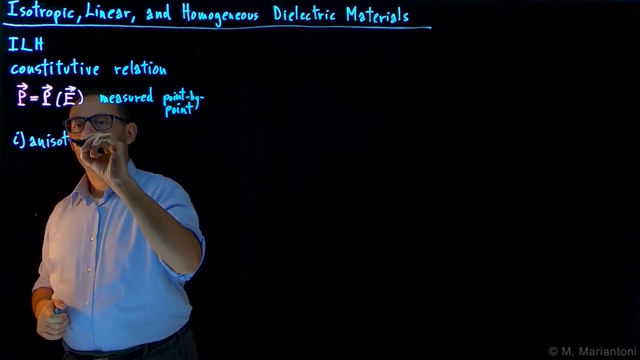 So how do we do that? First of all, let us consider the most general case, One Which is that of anisotropic materials, In contrast to isotropic materials, So anisotropic materials From Greek. this means that if I observe this material in different directions, 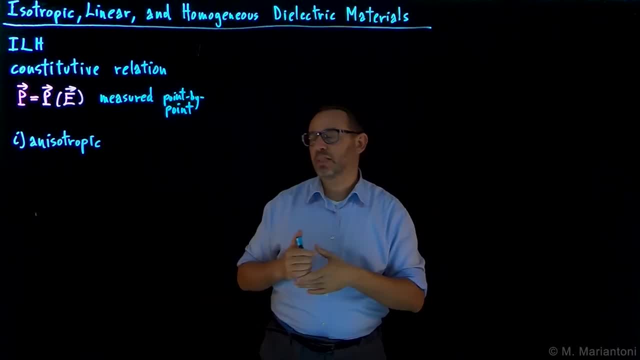 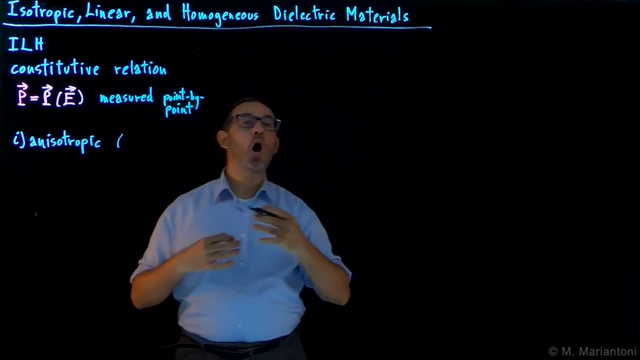 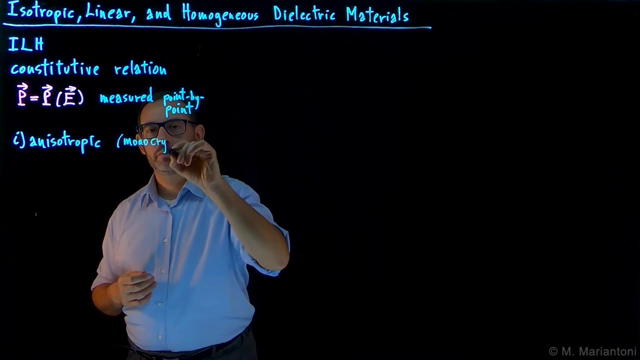 I see different arrangement of atoms inside this material, let's say, Or the molecules inside this material. So, for example, an isotropic material is a monocrystalline material Or single crystal. So how do we make a single crystal material? 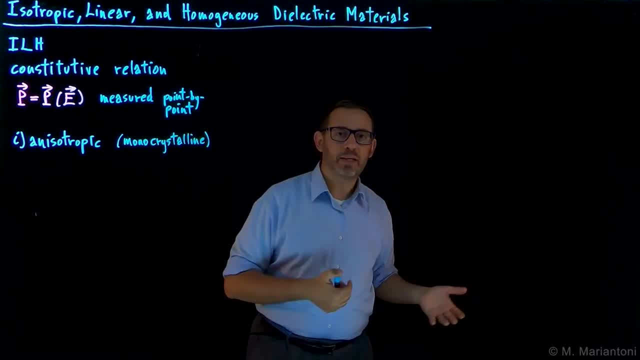 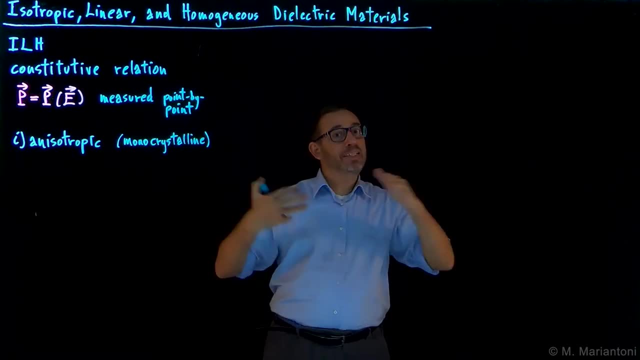 For example, by means of MBE, Molecular Beam Epitaxy, Which is something we use, for example, sometimes to make samples for superconducting devices. It is, of course, a very nice material because it is a single crystal, But the drawback is that it is harder to explain mathematically because it is anisotropic. 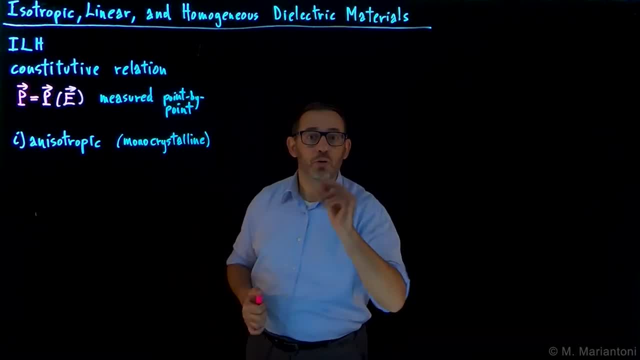 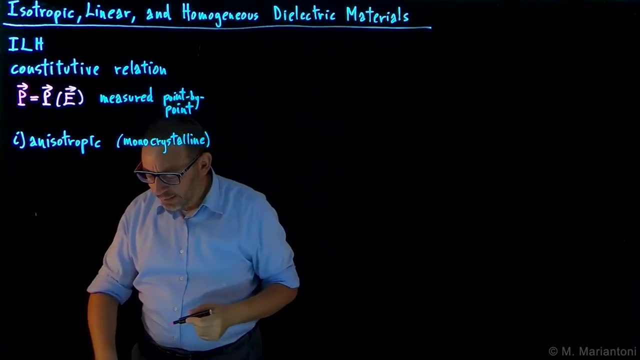 And why is it harder? Because in this case we need to use a second order tensor, As we have seen already for Ohm's law. Ohm's law in PHIS 242.. So we need a second order tensor, which in this case is for P. 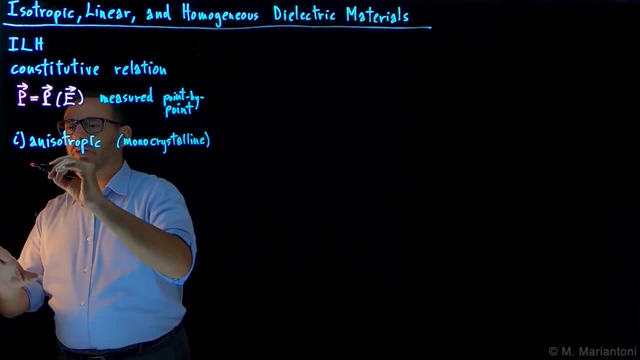 And so it would look like it is a 3x3 matrix. So first of all we need the input, which is the components of P, Let's say in a Cartesian coordinate system, Px, Py and Pz, And then we will have a matrix which is our second order tensor. 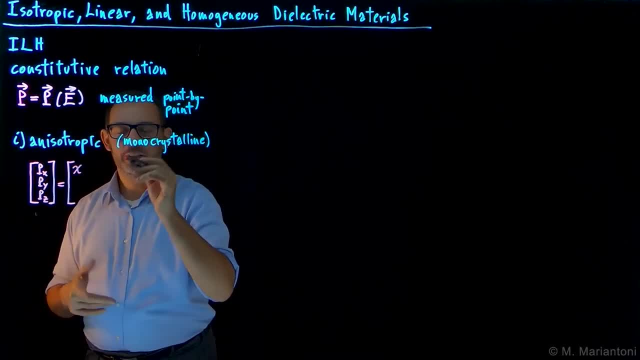 With components such as: let's call them chi. We will define chi, in this case, chi. we will define chi more in detail in a few minutes. chi, xx, chi xy, chi, xz, etc. chi, yz and finally, all the nine components. 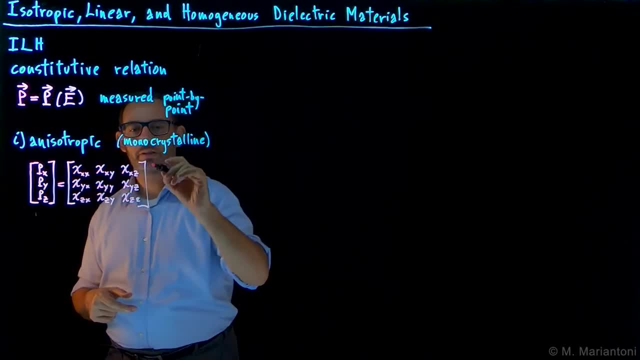 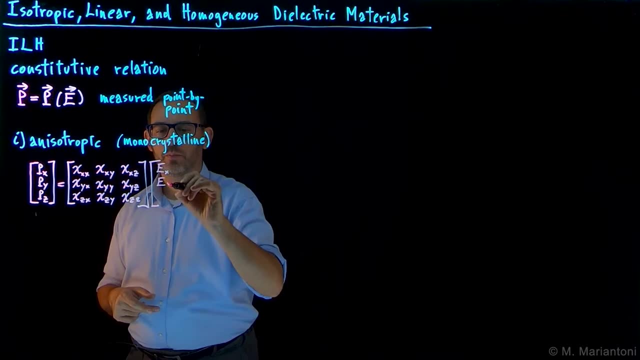 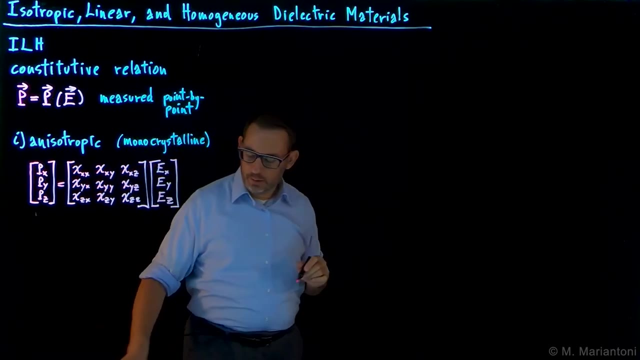 So we will have a matrix of this second order tensor. This gets multiplied by the components in a Cartesian coordinate system of E, Ex, ey and ez. We also have seen second order tensors in PHIS 342 when we studied a dipole in an external field. 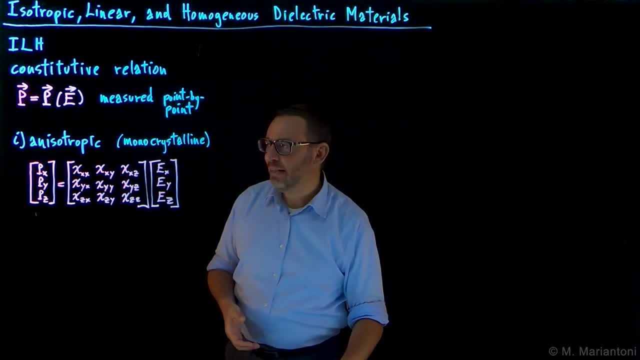 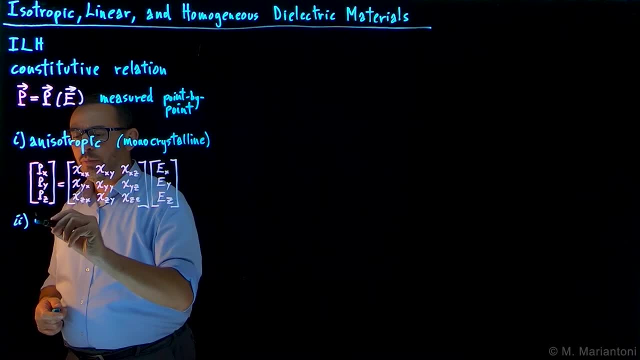 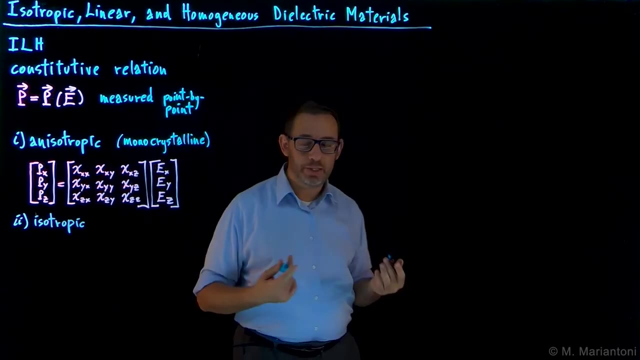 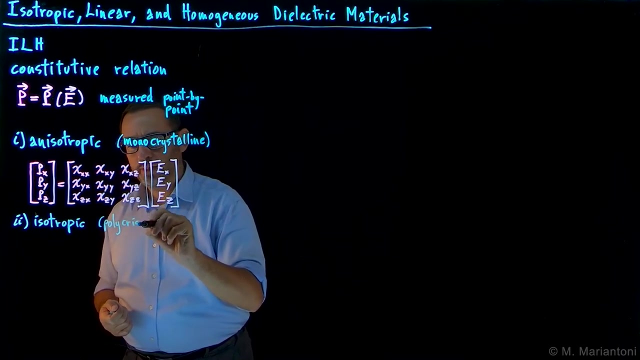 Okay, so this is fairly complicated. Luckily, in most cases, we will not encounter anisotropic materials. Instead, we are going to encounter isotropic materials. So what are isotropic materials? These are polycrystalline materials, amorphous materials and liquids. 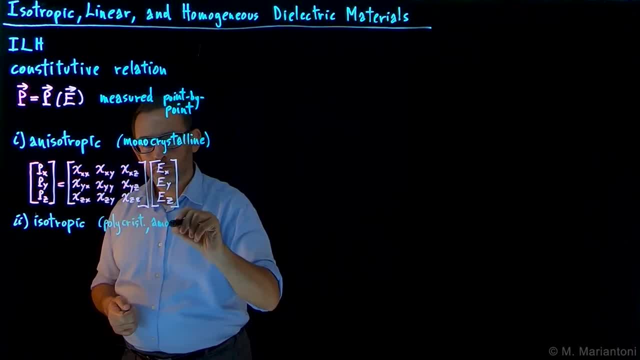 Polycrystalline amorphous liquids, etc. Okay, in contrast to monocrystalline materials, These are more common, in fact, in real life, And so in this case, the relationship between P and E gets significantly simplified. 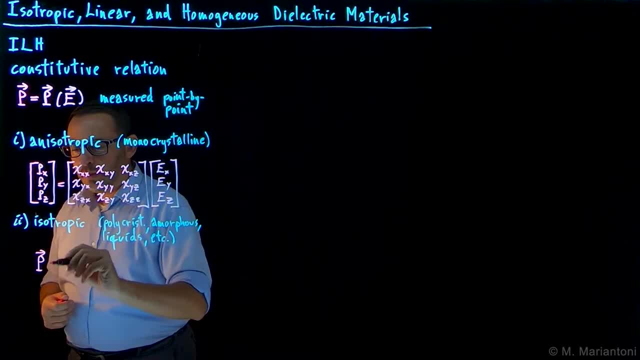 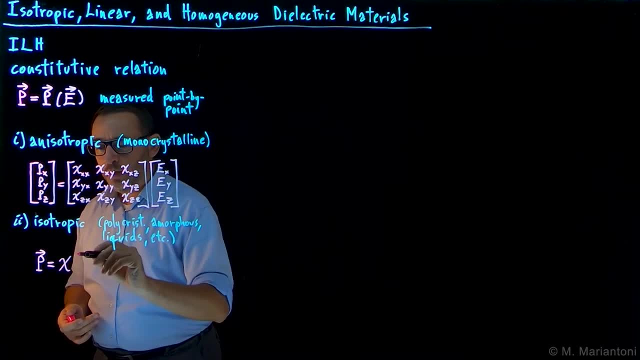 and it becomes P vector- happens to have the same direction as E by means of a constant of proportionality which, again, we call chi. This chi, in the case of isotropic materials, is still pretty complicated. It can be a function of the P vector. 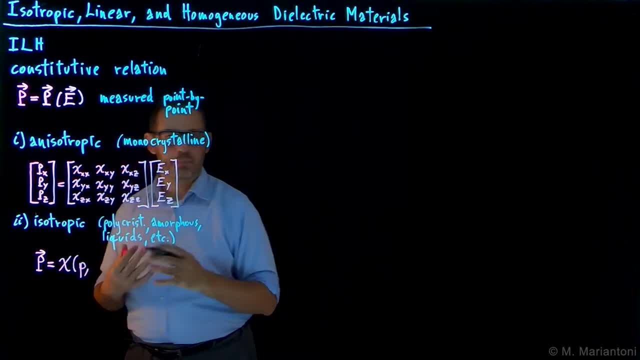 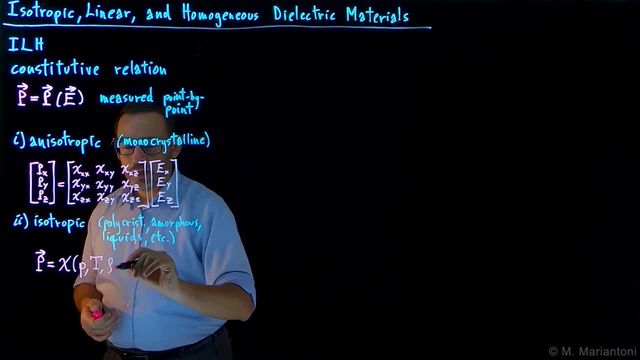 Pressure at which the material is, in this case for pressure is- prepared, can be a function of the thermodynamic temperature capital T at which the material is operated, and is a function in general of rho m, which is the density of mass for this material. 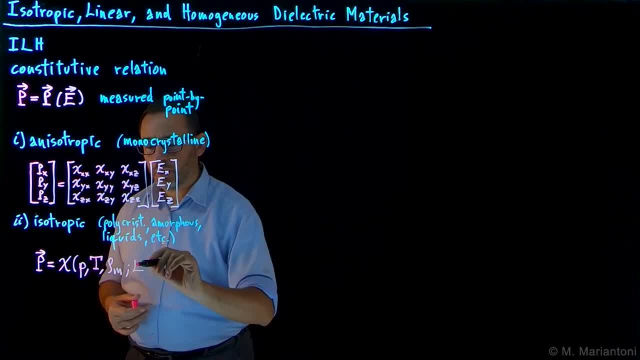 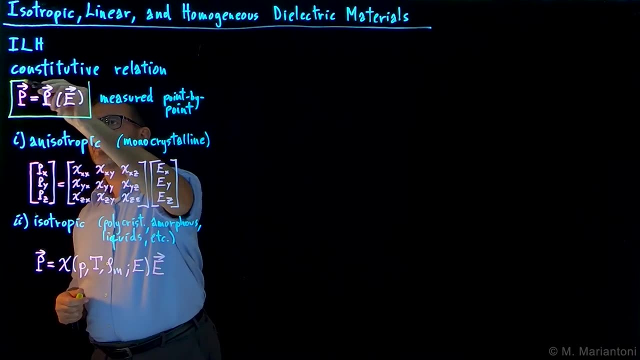 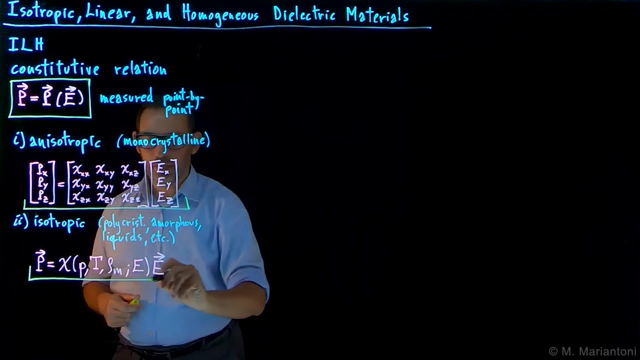 In addition, most importantly, it is also a function of the amplitude E, the intensity of the electric field. All this constant gets multiplied times E vector. So this is the most general case, This one is the tensor case And this is the isotropic case. 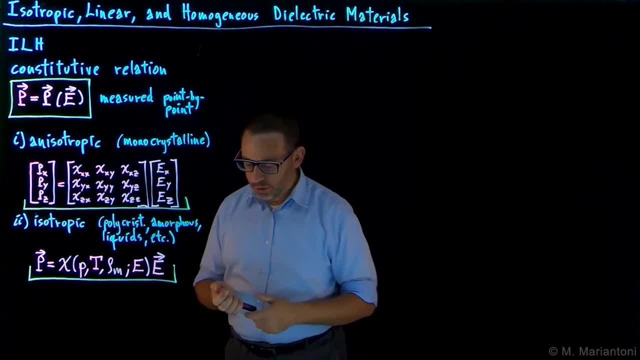 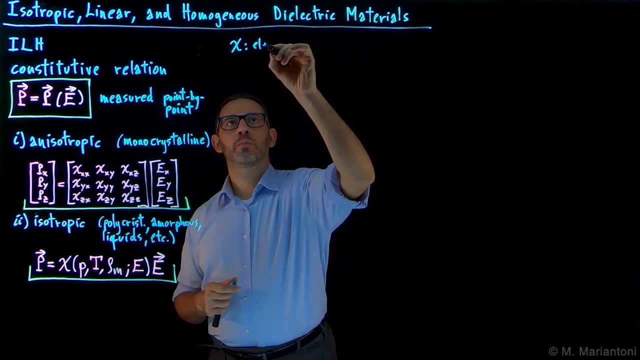 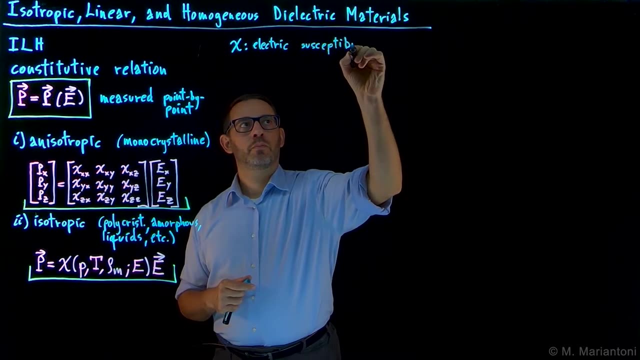 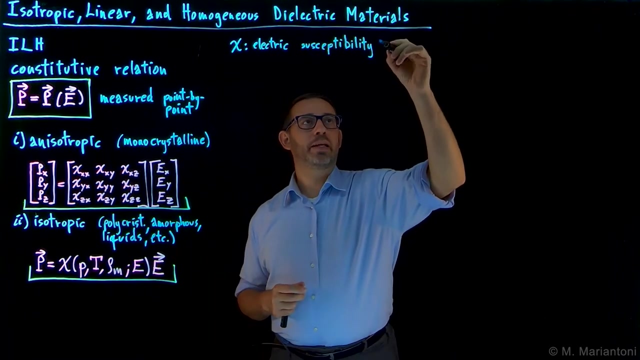 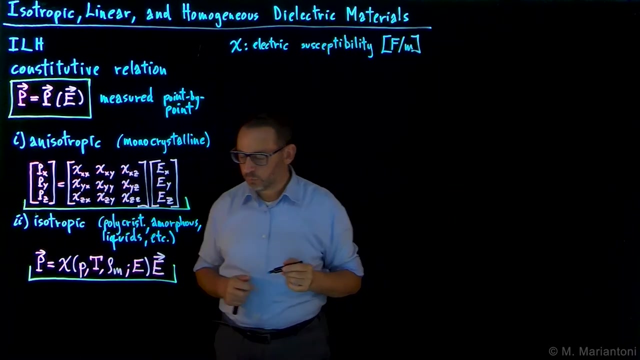 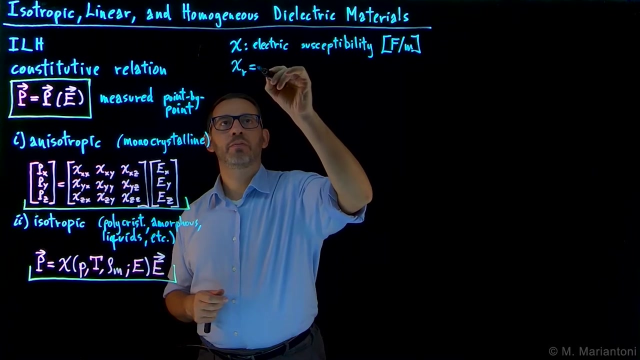 Now let's give some names. This quantity, chi, is called electric susceptibility. The units of the electric susceptibility in SI are farad, divided by meter SI units. In addition, we can also define XIR, a relative susceptibility which is given by XI renormalized over the electric constant of vacuum epsilon naught. 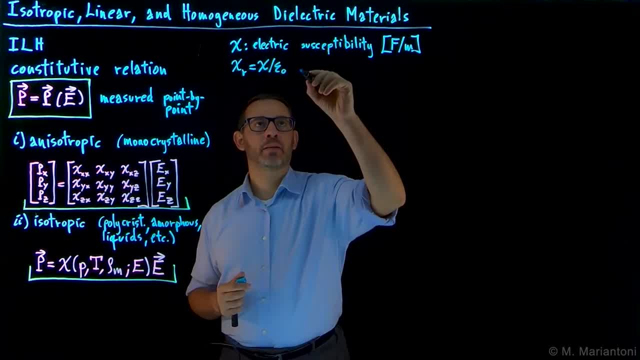 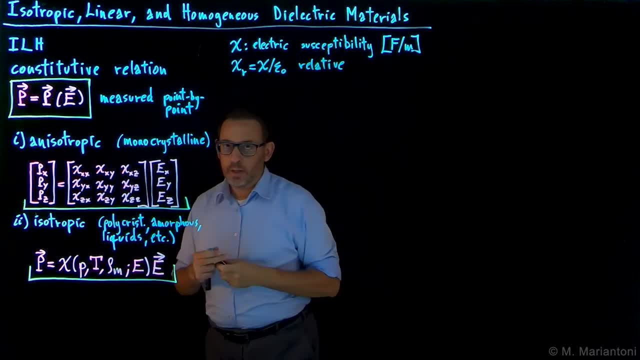 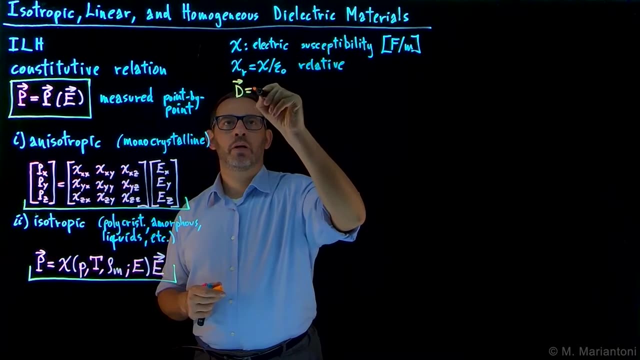 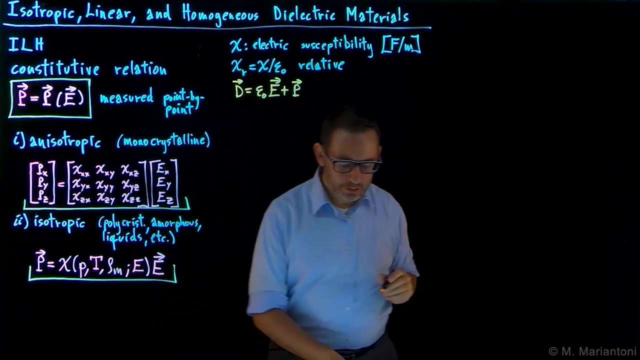 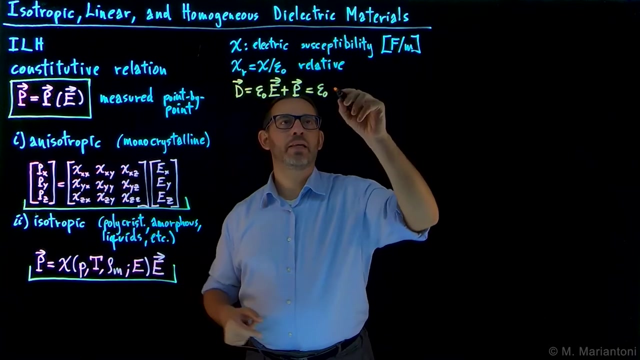 So this is the relative electric susceptibility Relative. Relative to epsilon naught Vacuum, that is. Now we know that D can be written as epsilon naught E plus P. Therefore, using this case of isotropic materials, we can simplify this expression. that becomes epsilon naught E plus chi E. 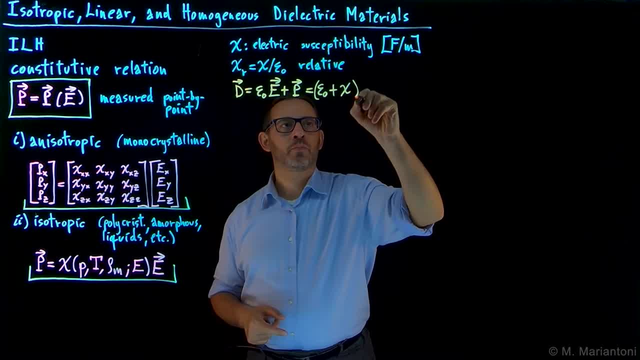 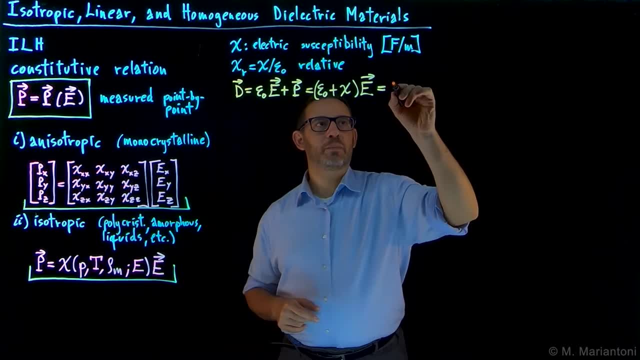 So it's epsilon naught plus chi, function of all these quantities, so this times E. This typically is written as epsilon, which again I'm not going to write it in this specific case, but the function of pressure, temperature, ram and E. 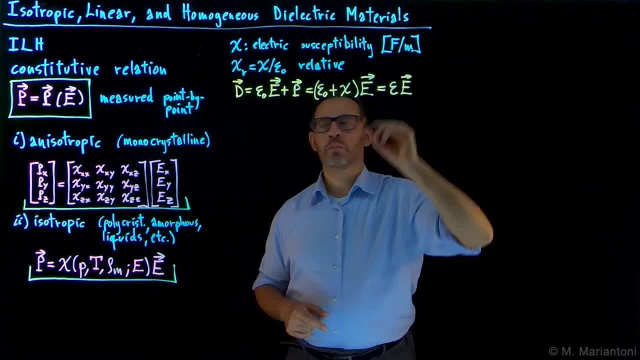 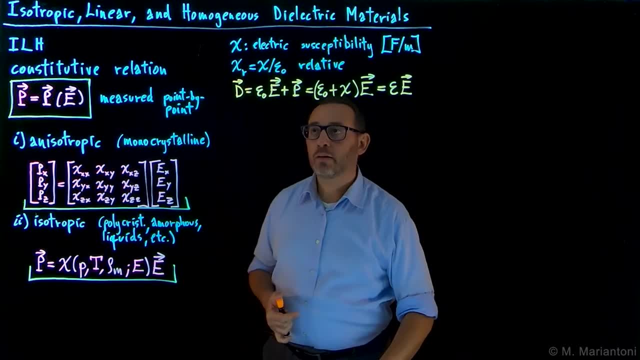 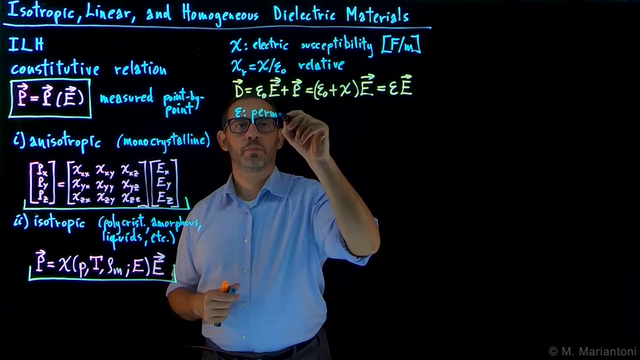 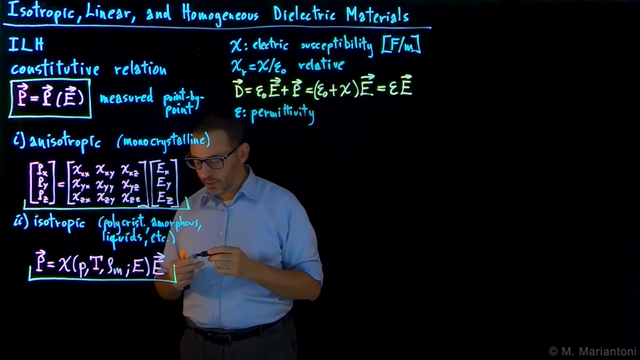 is epsilon times E, So D equals epsilon E. So this is a very important result. And so, this very important result, we define epsilon as the permittivity of the material. Where epsilon naught is the permittivity of vacuum, traditionally called the electric constant. 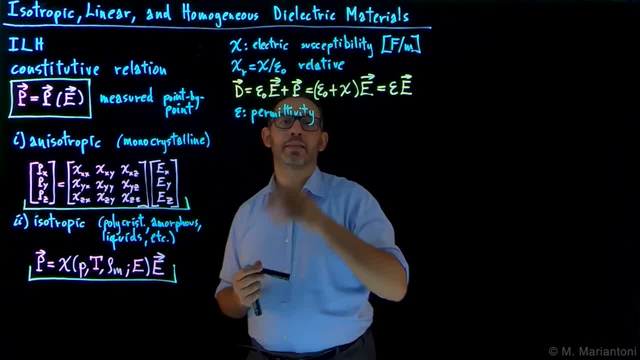 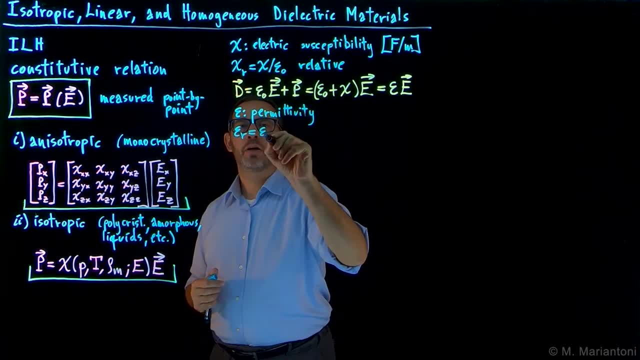 but that's an obsolete definition, And this is the absolute permittivity, whereas the relative permittivity, epsilon R, is defined as epsilon divided by epsilon naught, as here. Okay, So, given all that, how can we go now to even a simpler material? 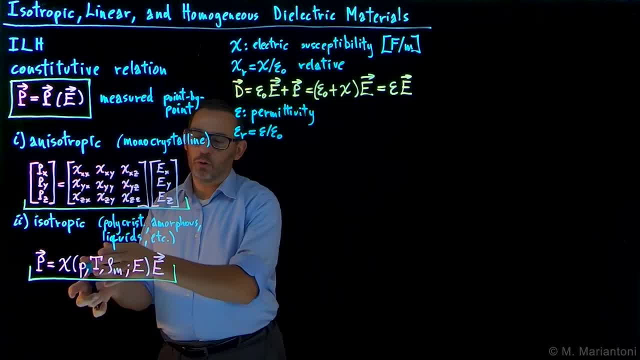 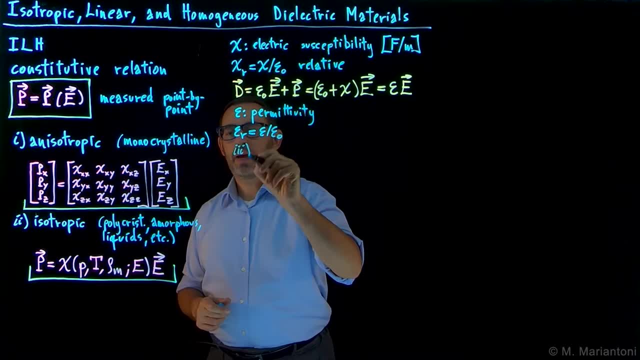 In order to make the material even simpler. clearly, we want to get rid of at least all these dependents from pressure, temperature and rho m, And so that type of material which is independent from pressure, temperature and rho m. 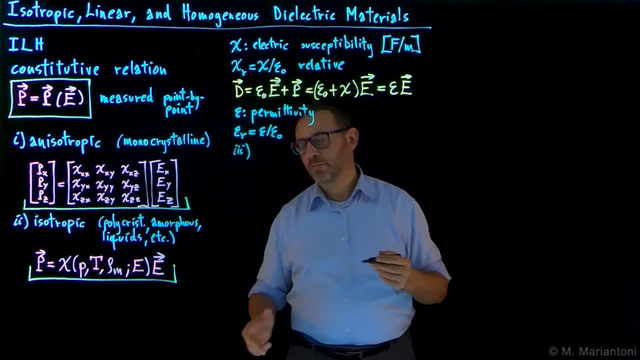 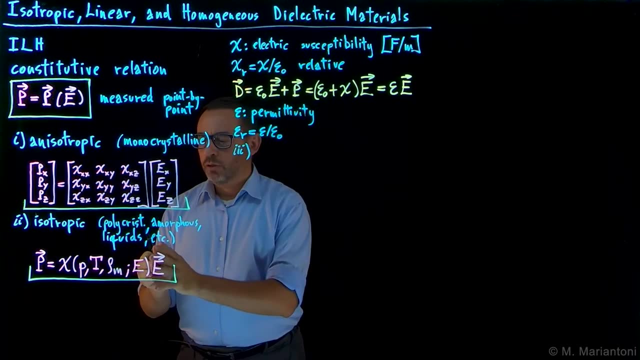 so where chi, the electric susceptibility, is independent from all these quantities, these parameters. it's called So before going there. so that's actually homogenous. the first step actually is to get rid of E. So then eventually we'll try to get rid of P, T and rho m. 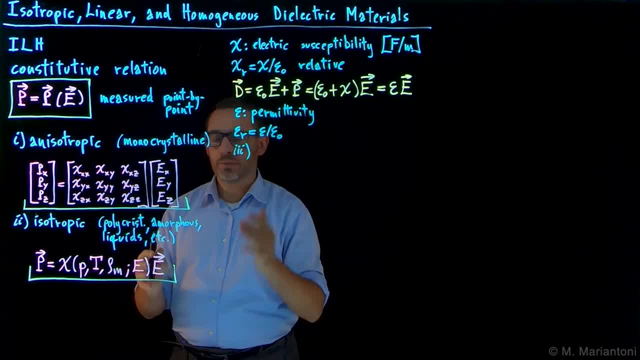 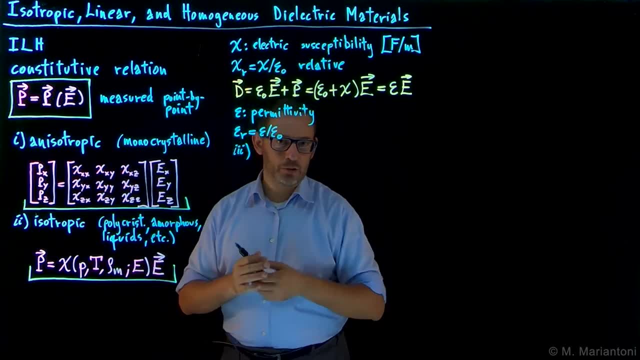 So the next step, the next material in this classification is a material which does not depend on E. So if the material is such that chi does not depend on E, and so I apologize, because first I start with P, T and rho m. 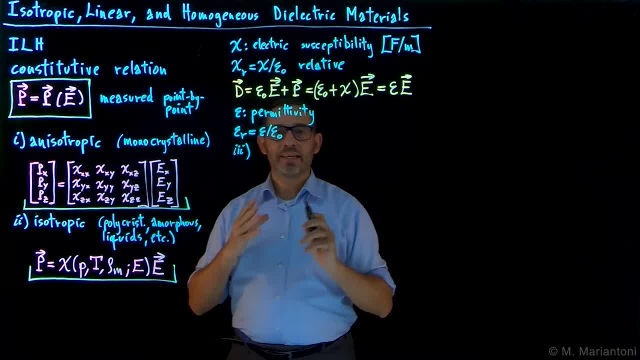 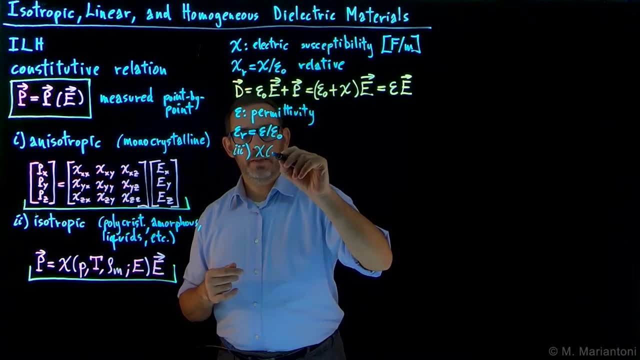 that's the next next step. So in this next step, chi is independent from E, which means chi is only a function of P, T and rho m. Eventually we also want to get rid of this, these parameters, But for now 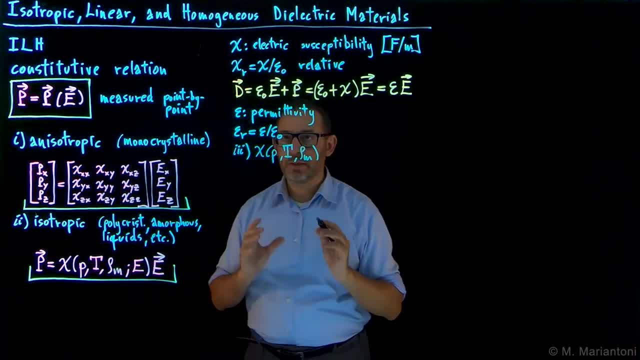 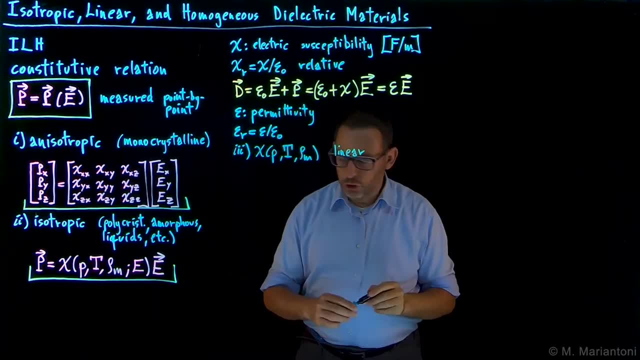 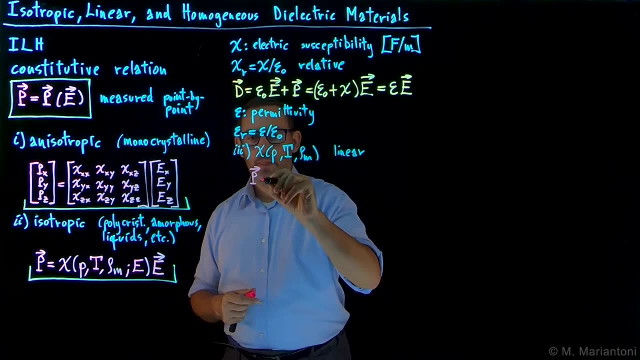 suppose that it does not depend on E. okay, It does not depend on the intensity of the electric field. In this case the material is said to be linear, So the constitutive relation for a linear material clearly becomes simply P equal chi. 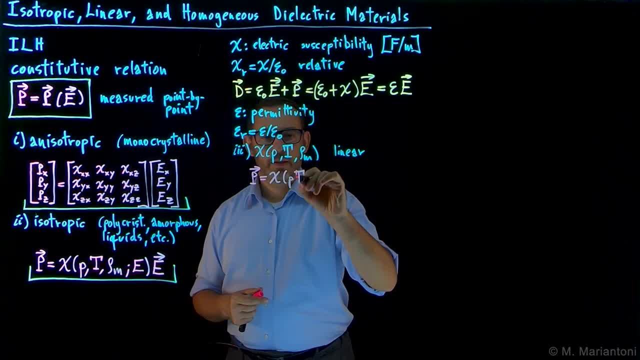 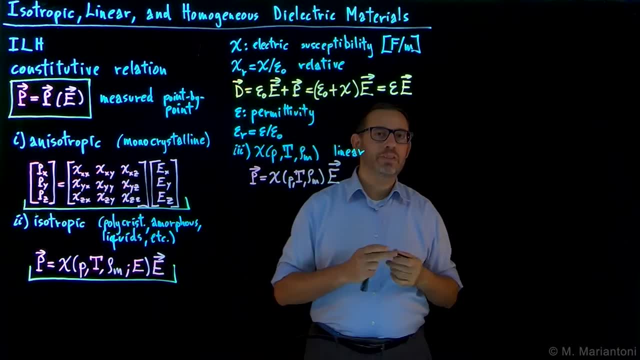 not function of E, It's just function of P, capital, T rho m times E. This is also true, of course, in real life. there is always a little dependence on E, So this is true also when the dependence from E is weak. 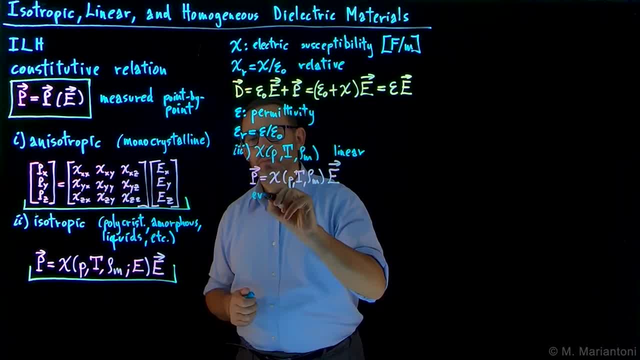 Okay, So even even when there is a weak dependence from E, then you can still use this constitutive relation. And how do we further simplify? Now we go to the last step, which is the one I kind of jumped to a few minutes ago. 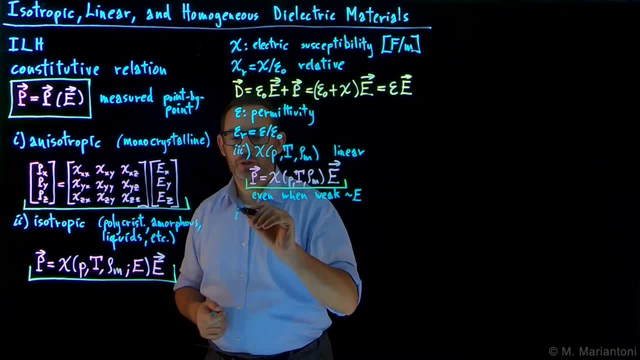 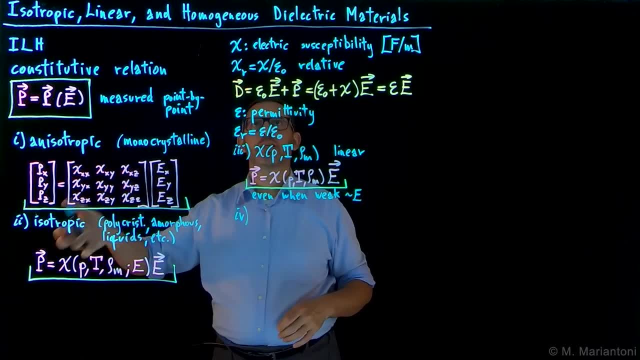 The fourth step and the fourth type of material in this classification, which is so. this is level of complexity or, if you want, or conditions we put on the material. So we start from the most generic: anisotropic, isotropic. 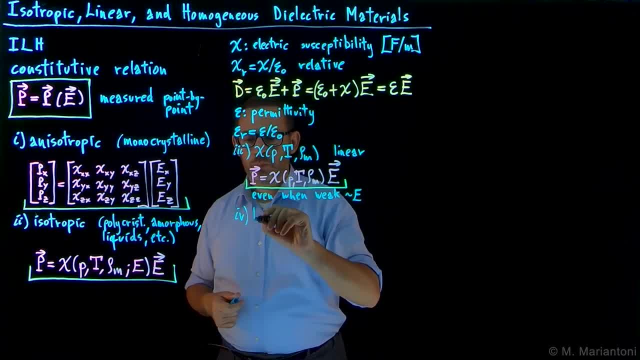 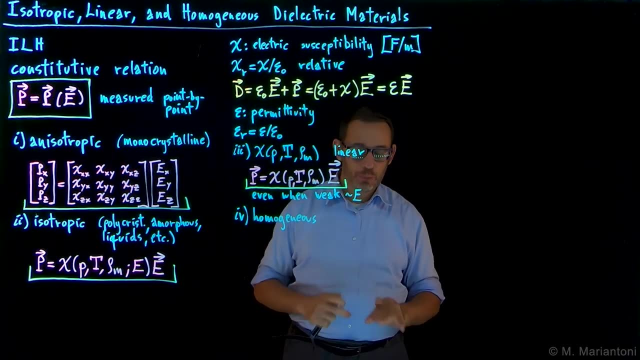 linear. and finally, we want to define a homogenous material. So as the words say homogenous, same everywhere from Greek. this clearly means that in this case, chi does not depend on anything at all, It's just a pure constant. 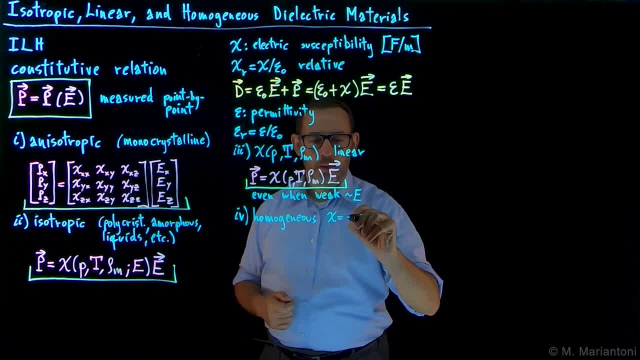 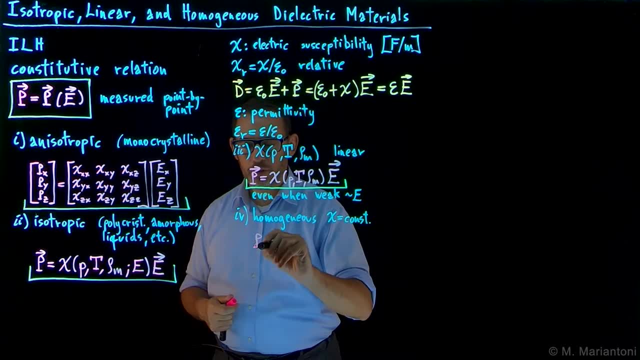 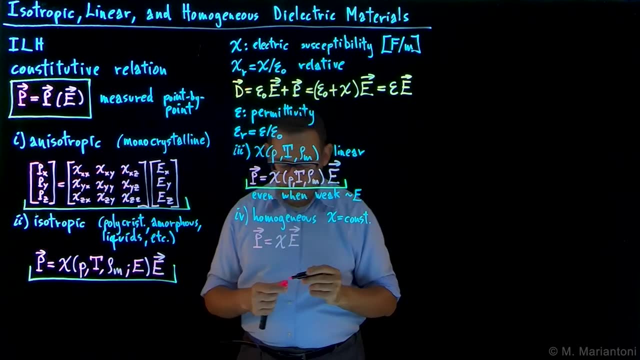 So in this case chi is just a constant. As such P, the constitutive relation becomes very simple: Equal chi times E. This is similar to Ohm's law, which we have seen in 242.. In that case we had a relationship between E and J. 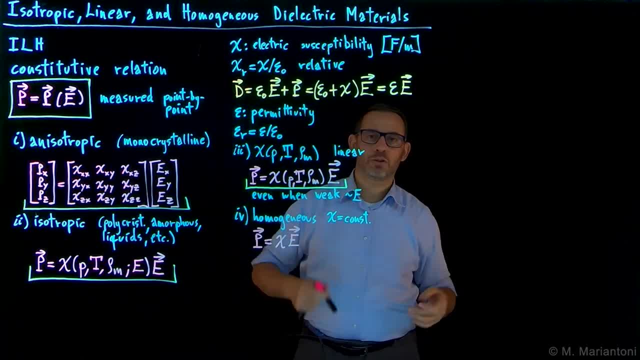 And in that case also we started from anisotropic conductors, where we had resistivity or conductivity which were in a tensor form, second order tensor, et cetera, et cetera. Eventually we also arrived at these homogenous materials. 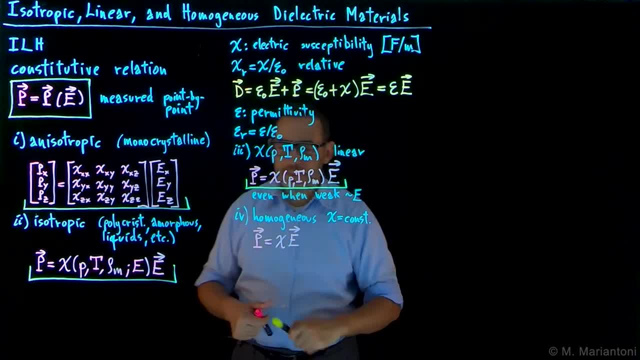 where the conductivity, the resistivity is constant. Same thing here. So this is the constitutive relation which mostly we're going to use in the next videos, in the examples we are going to do in the next few videos. So P is equal chi E. 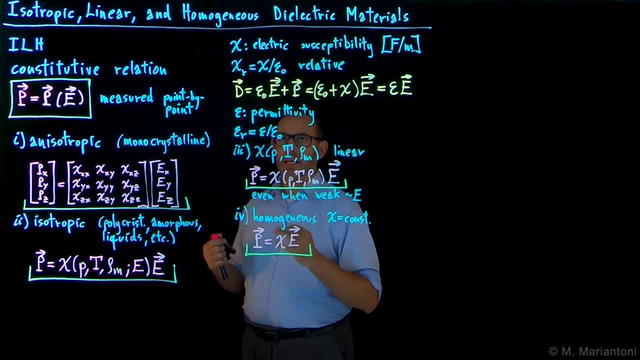 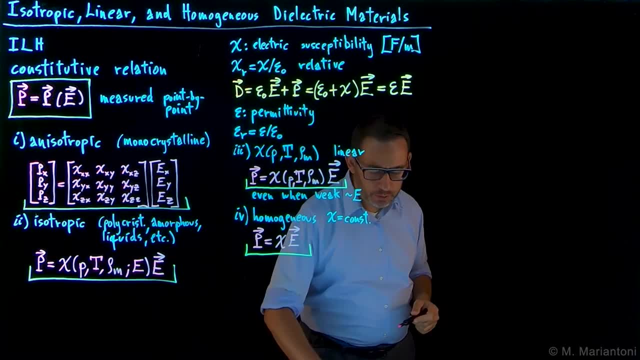 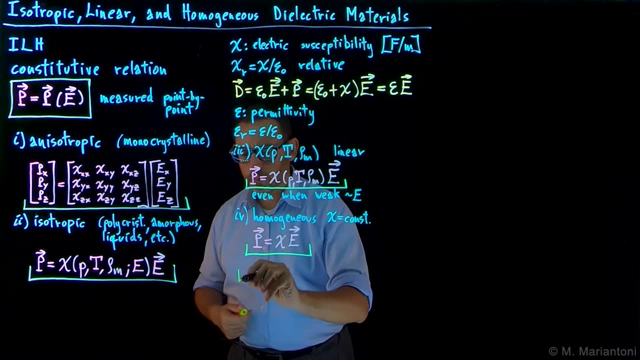 where chi E is the constant electric susceptibility of the material. Okay, So in particular it's worth investigating and I will let you do this in piazza. so a question which I have for you in piazza is: calculate the curl of B. 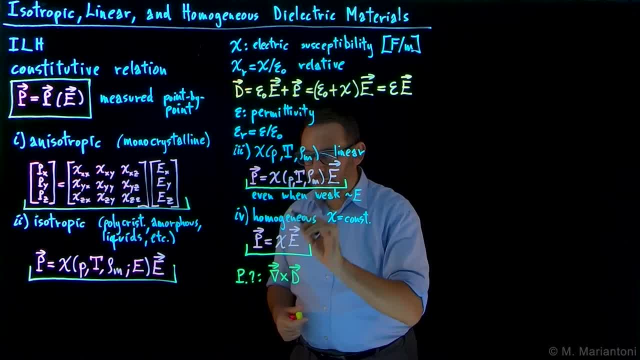 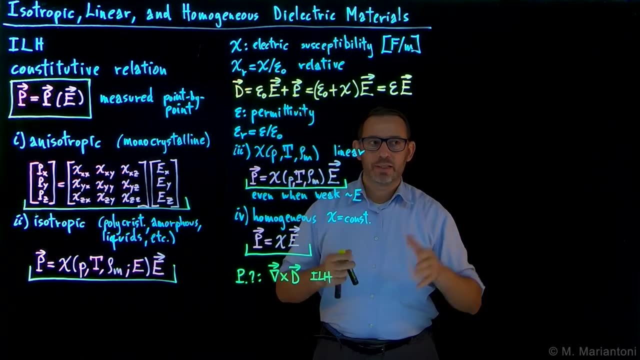 in presence of isotropic, linear and homogenous dielectric materials. So for ILH materials, what is the result of the curl of D? Well, normally you will find something interesting, but also you should think about the surfaces, what kind of behavior the electric field has to have. 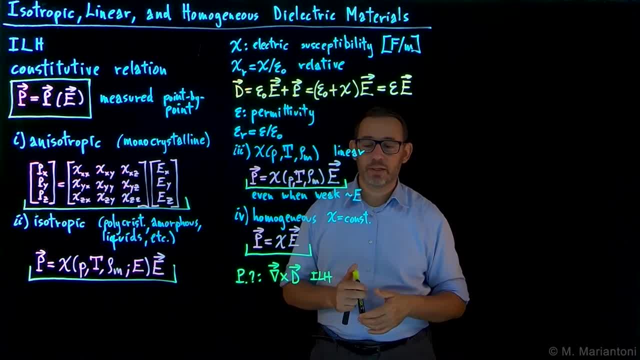 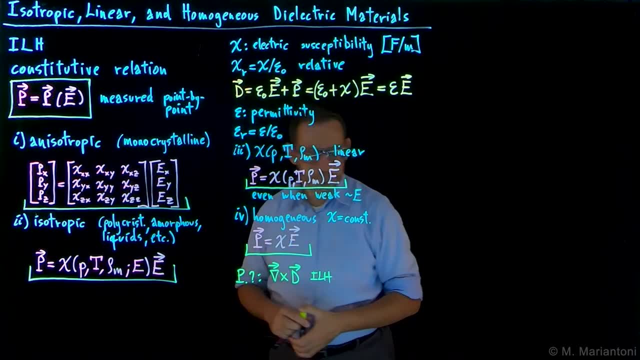 at the surfaces and the interface between the dielectric materials and vacuum, for example. But first of all, just use all these conditions to calculate the curl of D, That is for ILH materials. Okay, There is a sub definition which is worth reporting here. 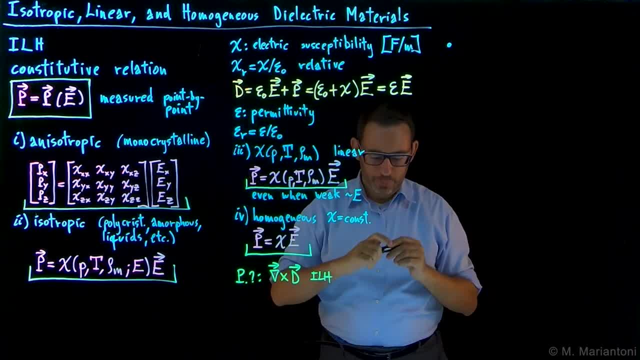 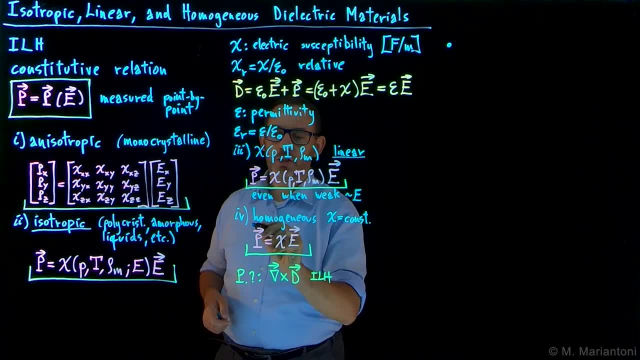 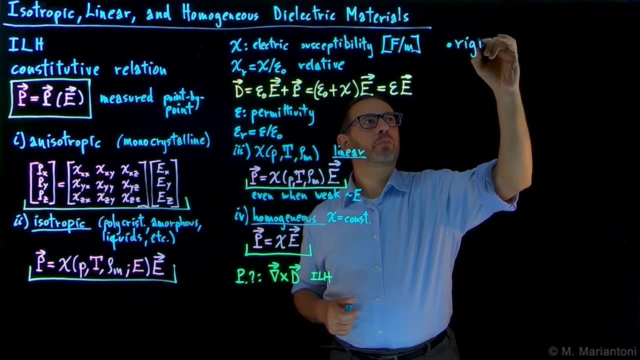 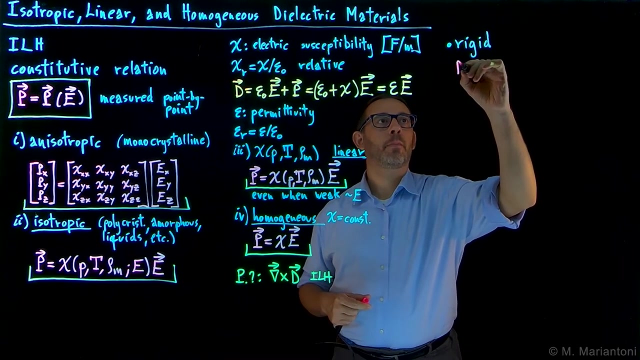 So we can have isotropic. Let me highlight all these key points: Isotropic, linear and homogenous dielectric materials. One extra special category is that of rigid materials. For rigid materials, it so happens that P is only a function of the external. 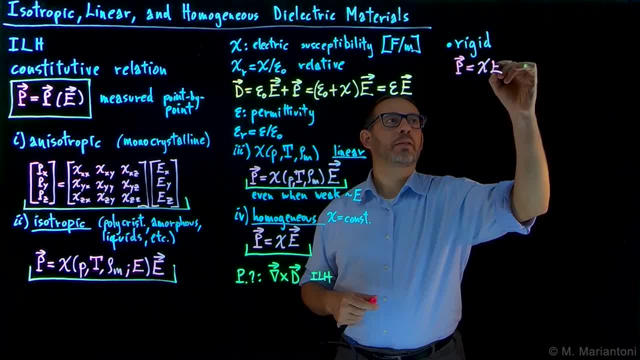 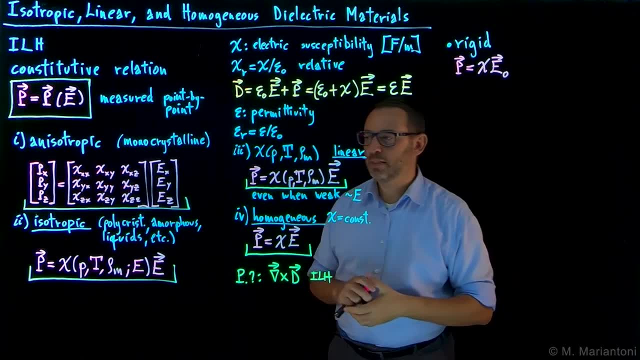 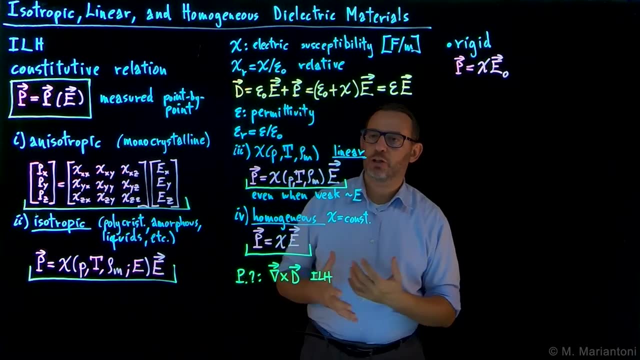 field E naught that generates the polarization. So these are rigid, So it doesn't depend on the polarization field, which also eventually is in this material. Okay, So what about this condition of linearity? Let's discuss a little bit about this. 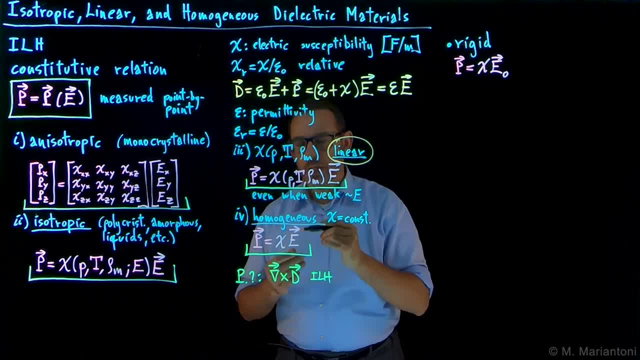 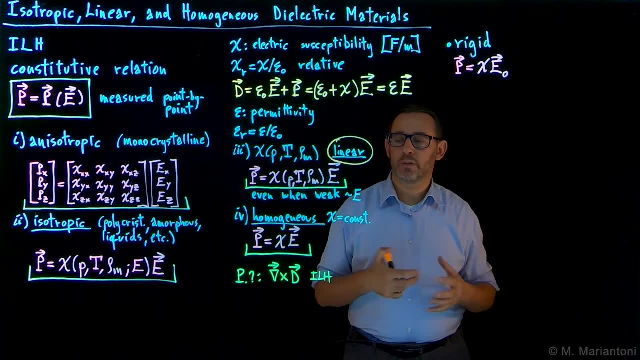 So, as I mentioned here, this relationship where chi only depends on pressure, temperature and mass density and the density of mass inside this material, It's true even when we have a weak electric field. How weak does it have to be? Okay, So if you start to crank up too much the electric field, 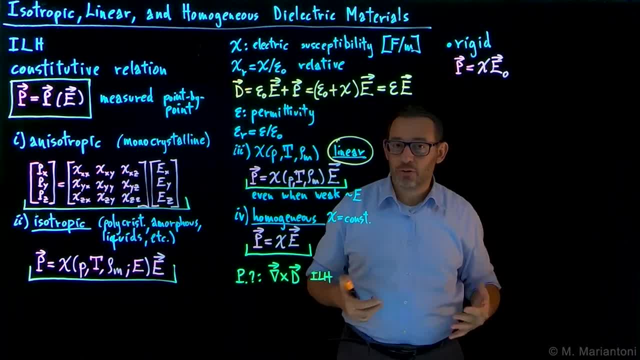 that generates the polarization. you eventually reach a so-called electrical breakdown. So things start to break and all these models also don't work anymore. So just to give you a sense of the relative permittivity as well as the electric background, the maximum electric field for a few materials. 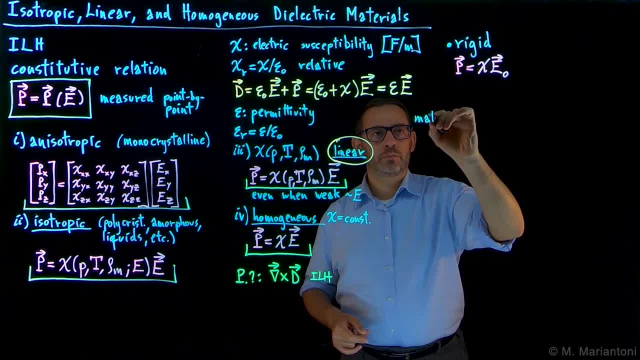 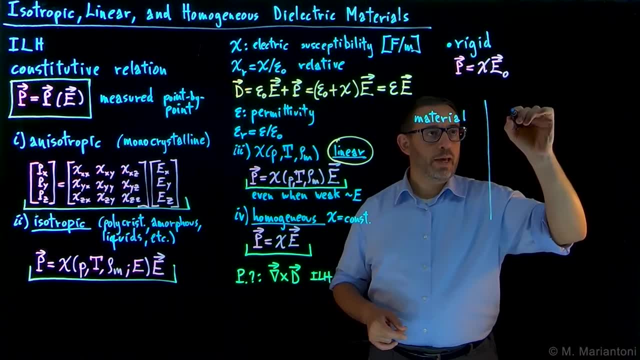 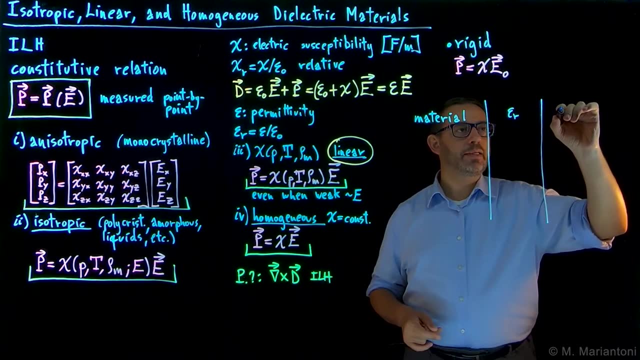 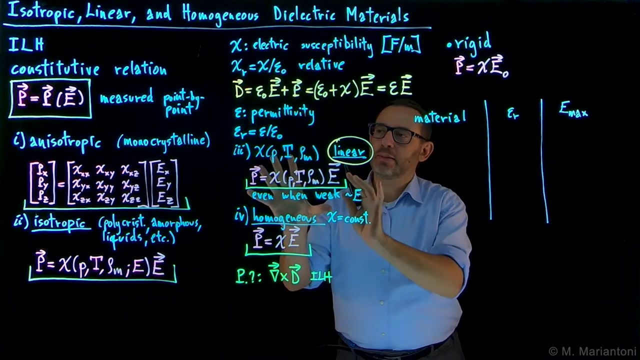 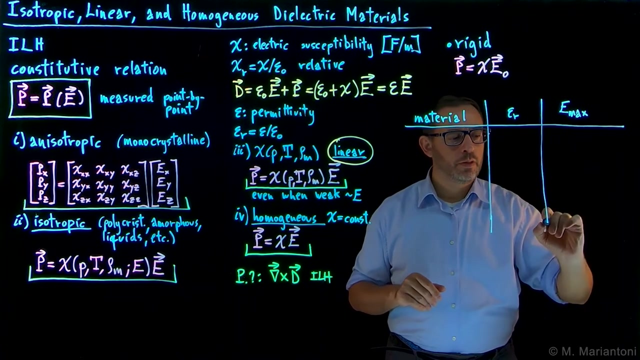 let's make a table here where we have material epsilon, r- relative permittivity of that material- and finally the E max, the intensity of the maximum field for which there is no electrical breakdown, And typically this linear condition can be used. 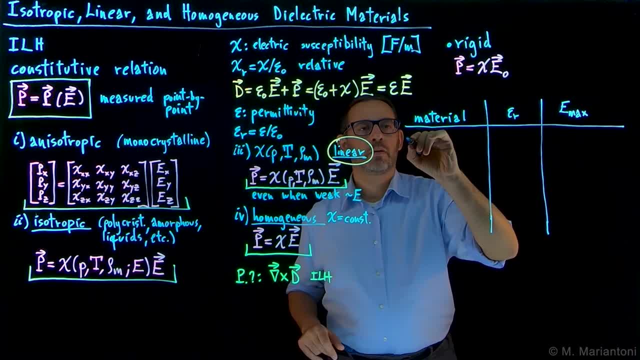 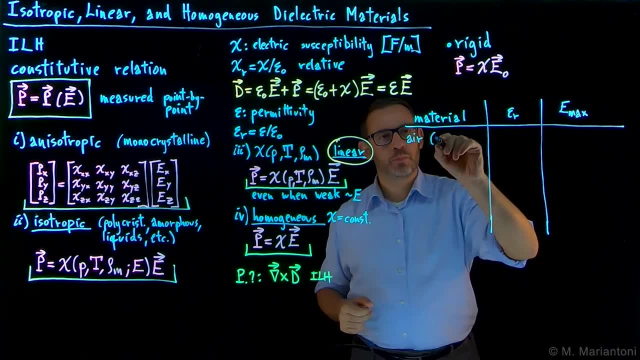 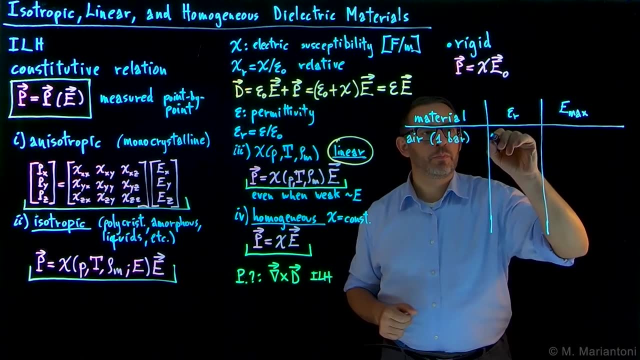 So, for example, if we consider air and let's say at a pressure, we are still in this condition. so there is pressure of one bar. Epsilon r is very close to one, like, almost like vacuum, Street zeros 59,. 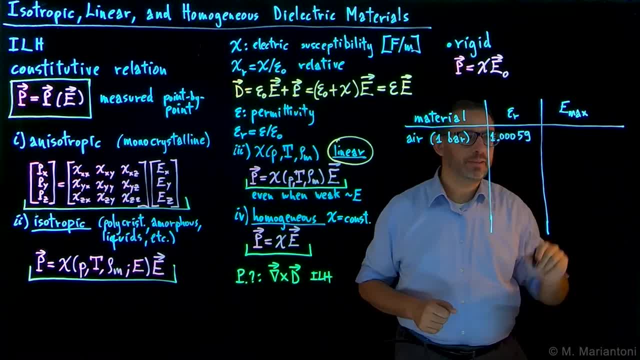 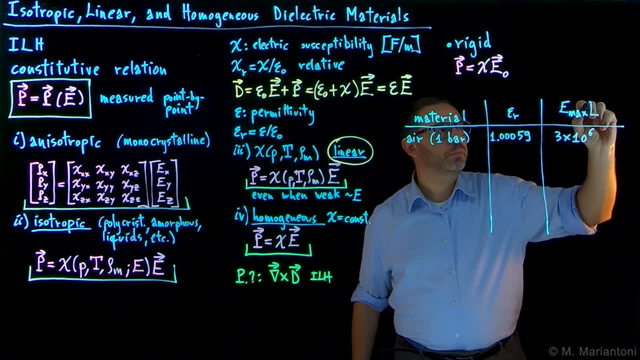 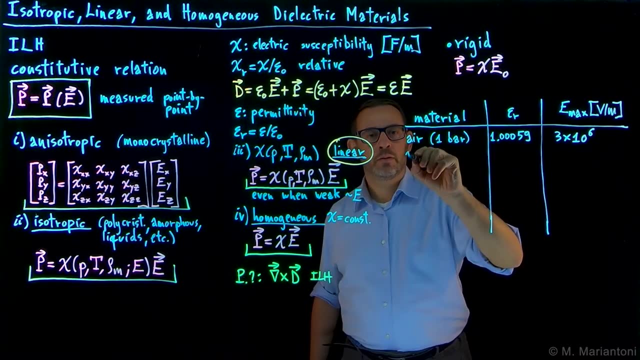 very close to vacuum. The E max is three times 10 to the sixth. What is the unit? what are the units of E max? Volt over meter, of course, Okay. What about air? So a different pressure, let's say 100 bars. 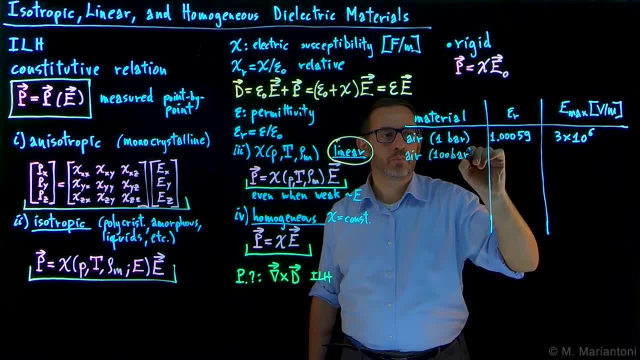 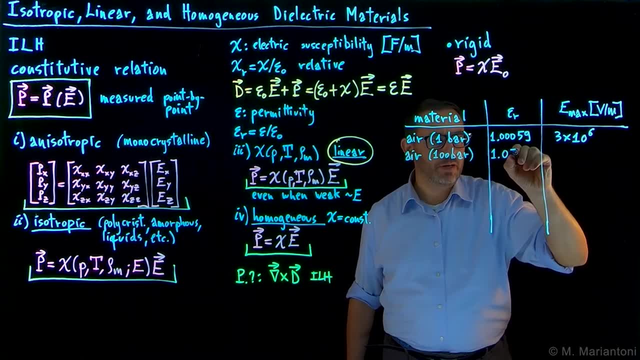 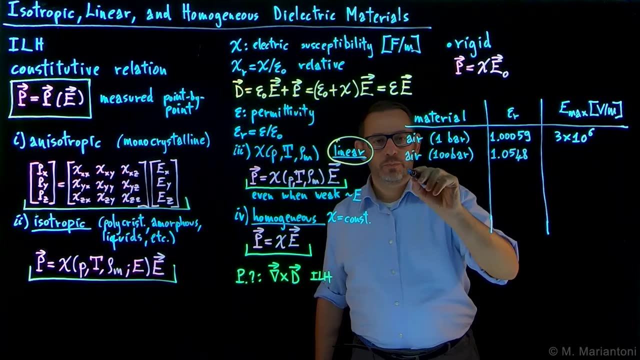 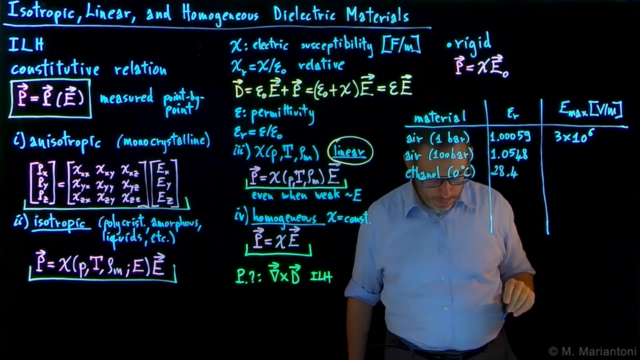 So we increase pressure a lot. Well, in this case, the epsilon r becomes slightly larger: zero, five or eight. What about ethanol? And let's say, ethanol at zero degrees Celsius, 28.4 is epsilon r. What about nylon? 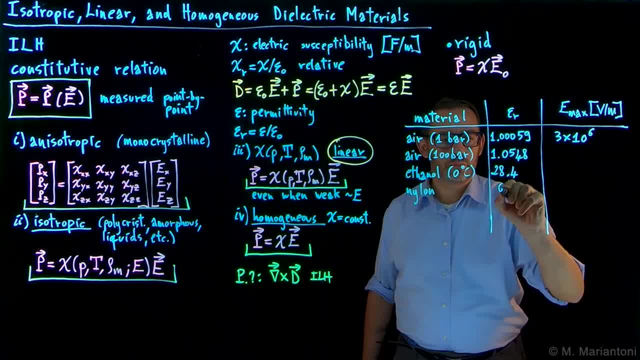 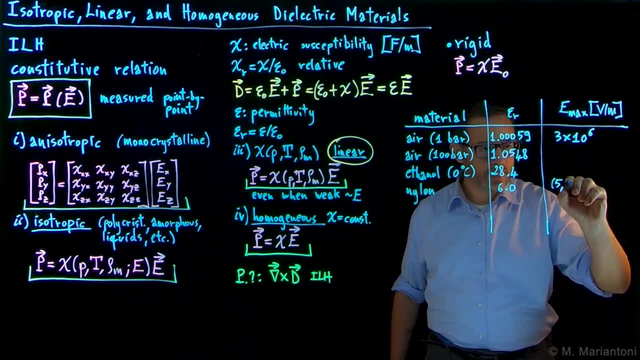 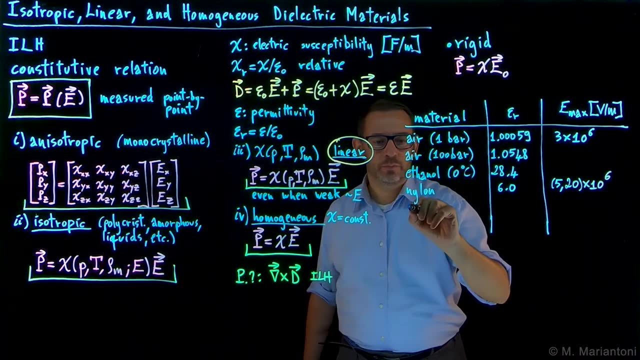 In the case of nylon, we have 6.0. And in this case the breakdown happens between five and 20 times 10 to the sixth volt per meter. Finally, what about glasses? Various type of glass. So in this case, 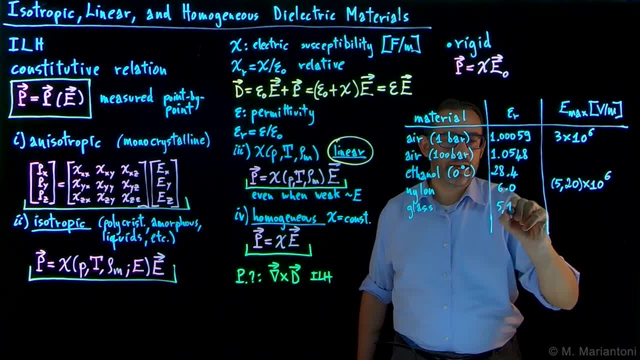 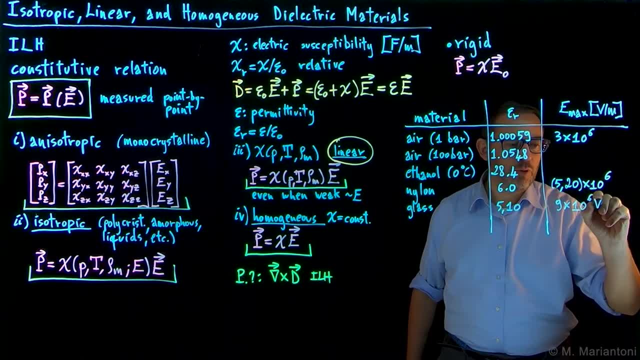 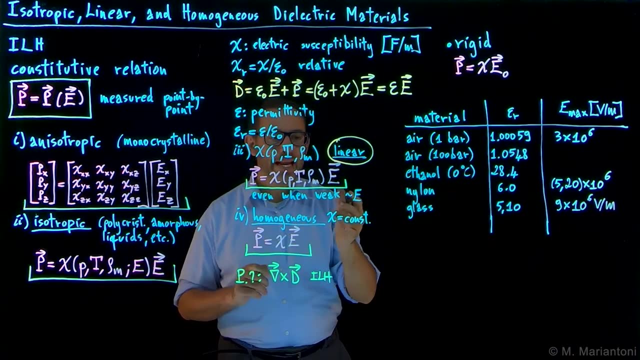 epsilon r is between five and 10. And the breakdown is approximately nine: 10 to the sixth volt meter. So if you are well below such values- 10 to the sixth volt per meter- typically the linear condition is good. You can forget about the. 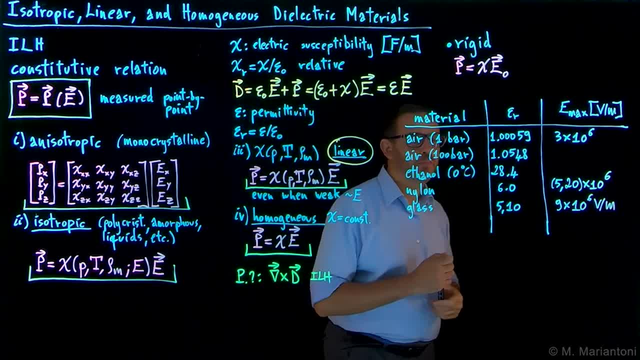 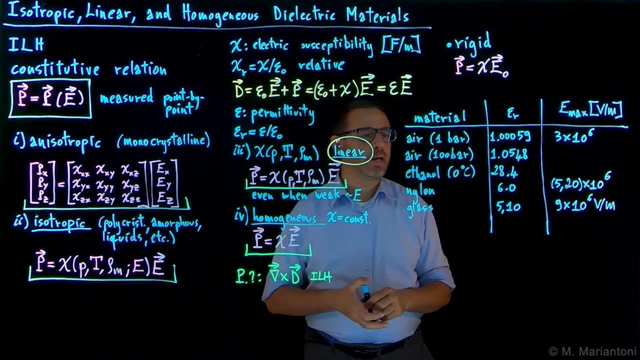 can neglect dependence on the intensity of E. Just to give you an idea, for example, silicon has an epsilon r of about 10, similar to sapphire. Tethylon is approximately three, and so on and so forth. Vacuum, of course. 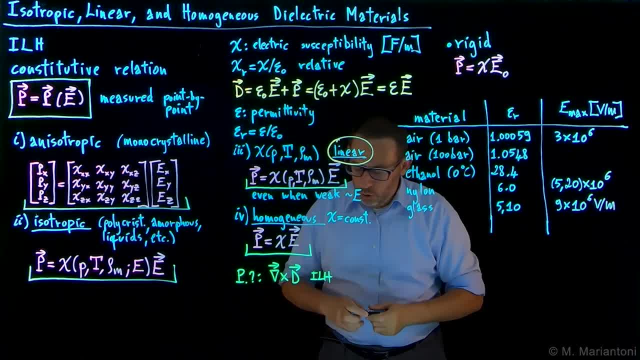 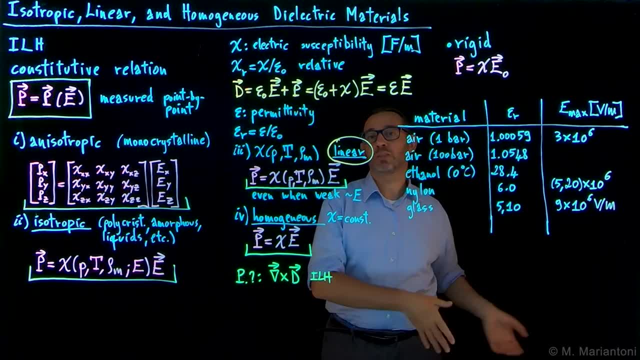 is one by definition if you have pure vacuum. Okay, So to summarize this video, we introduce a classification of materials. In particular, we introduce the materials we are going to study in the next videos. These are one of the most important type of materials. 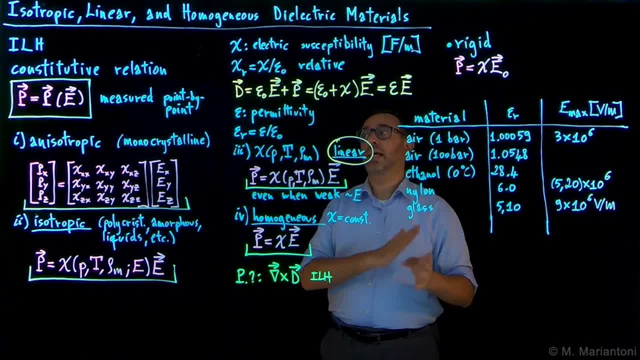 which are isotropic, linear and homogenous dielectric materials- ILH. In order to define ILH materials, first of all we need to introduce a constitutive relation Like in Ohm's law. we wanted the law between the electric field. 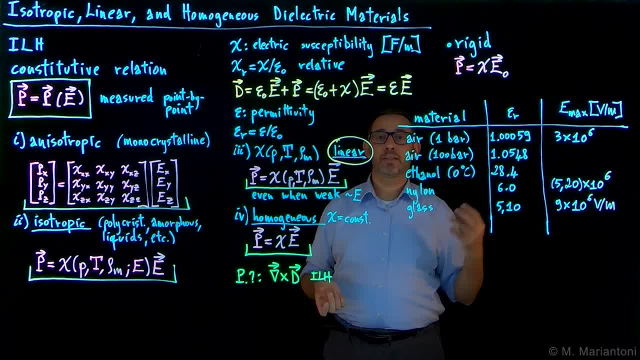 and the current density J. Here we want the relationship between P and E, which is measured experimentally point by point within the dielectric material. If I have a nonisotropic material like monocrystalline, then I have a tensor relationship. 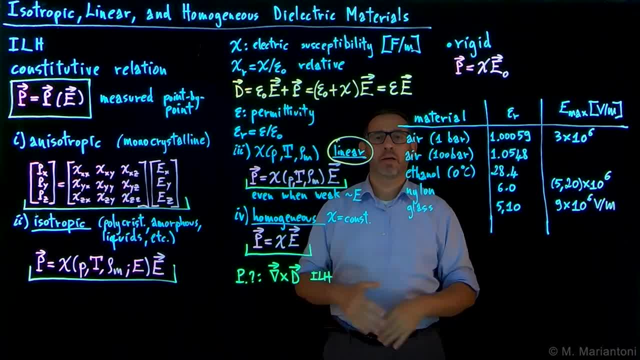 between P and E Very complicated. If I choose to have, if I manage to get an isotropic material. isotropic means same everywhere I look into it. from Greek it means the same everywhere I look into it. from Greek, it means the same everywhere I look into it. 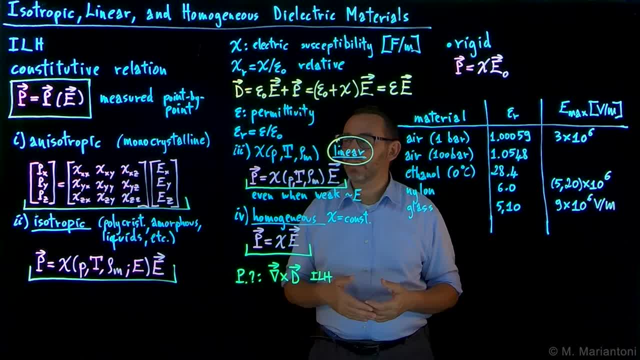 from Greek it means the same everywhere. I look into it from Greek. for example, polycrystalline on amorphous materials or liquids, polycrystalline on amorphous materials or liquids, then P is proportional to E. 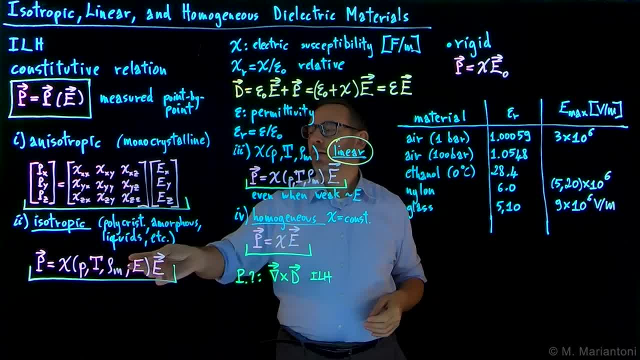 with a proportionality quantity, then P is proportional to E, with a proportionality quantity, chi, which depends on pressure. which depends on pressure? well, the pressure of the material, temperature, and rho m and as well and more importantly, 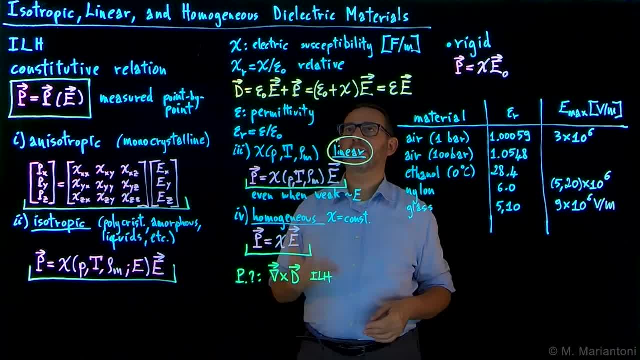 the electric intensity E. Chi is called the electric susceptibility unit sparad over meter. We can define a relative one by the definition of D. In this case, we can divide D by epsilon E. We can divide D by epsilon E. 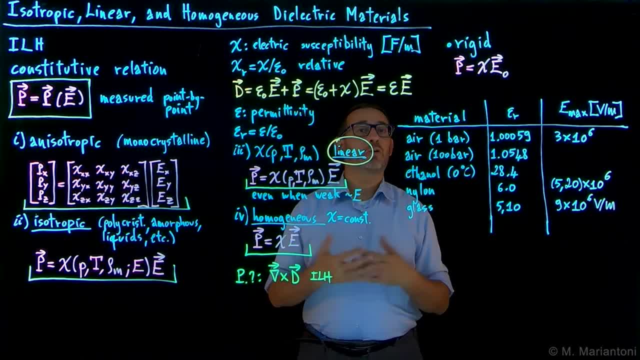 and we can choose it by the differential of the temperature of the material. what that means- very important relationship to be used later on in the next videos- epsilon is the permittivity of the dielectric material. also here i can define a relative one. what about linear materials? linear? 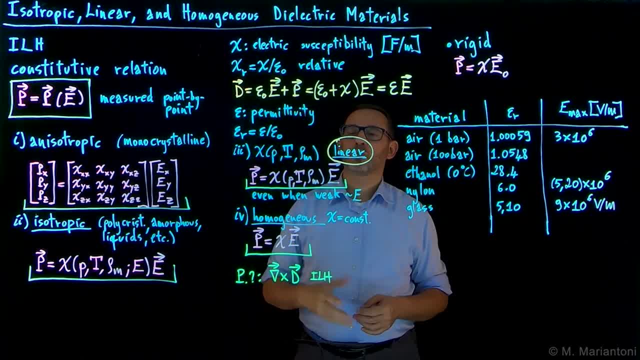 materials is when i have a weak dependence of chi over e, so weak, for example. here i give an idea of how weak it has to be. something like typically for these materials: less than 10 to the 6 volt per meter. you are good to go. you can neglect dependence on e, which means chi depends on your. 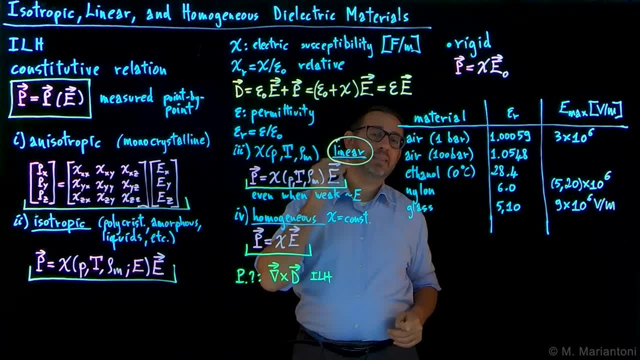 pressure, temperature and mass density. homogeneous materials. chi is constant, so we don't have, we just have a constant which does not depend on any parameters. and so this is the simplest constant relation, which tells us that p is proportional to e by means of the electric constant susceptibility. 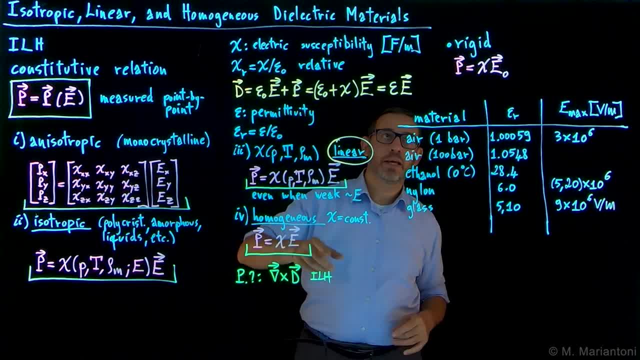 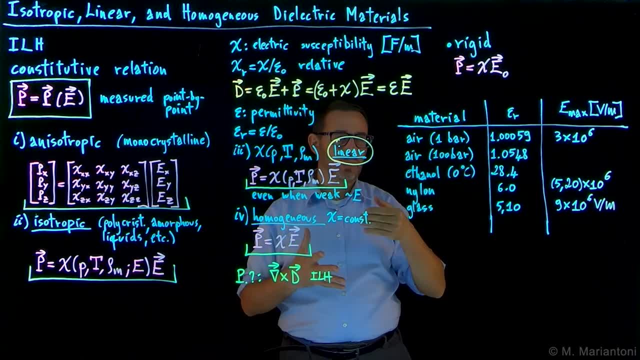 i asked you to calculate the curl of d under these conditions of ilh. a subset of ilh materials is rigid where p is equal to chi- e naught. it only depends on the external field, e, naught, not on the polarization field e, p. and here i just gave you an idea of